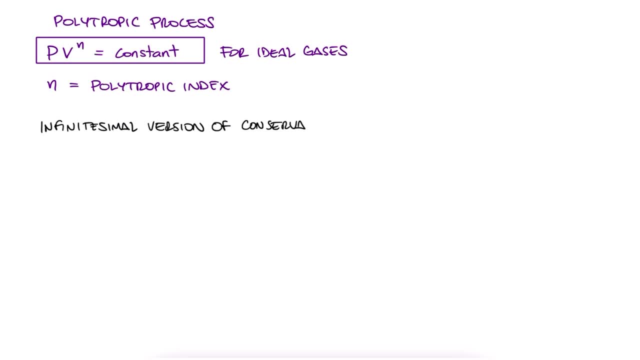 this. We know that for infinitesimal changes, our energy conservation equation, or first law of thermodynamics, results in: delta Q equals to du plus delta W. The heat can be written as mc, dt, with C being the specific heat at constant pressure, Cp, or constant volume, Cv, depending. 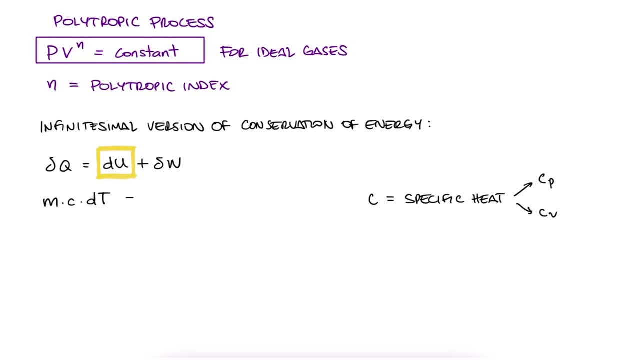 on the process and therefore indetermined for now. And du is equal to mCv dt. from the definition of what Cv is, The infinitesimal work is just Pdv. We can simplify this equation as mC minus Cv dt equal to Pdv. For an ideal gas, Pv equals to mRt. The differential form of this equation would be: 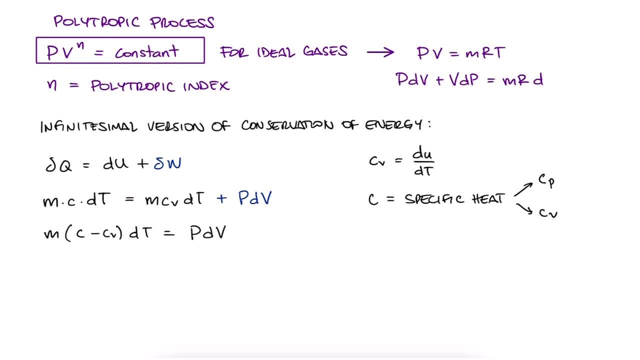 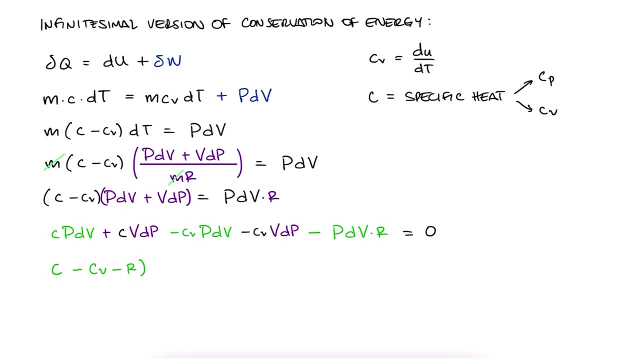 Pdv plus Vdp equals to mR, dt. We can solve for dt and substitute it in the conservation of energy equation. Since the mass term cancels, we can now multiply by R on both sides, then distribute the parentheses. and since in the last lecture we proved that Cp equal to Cv plus R, 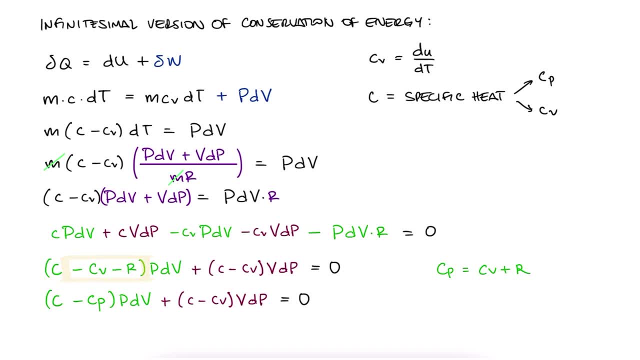 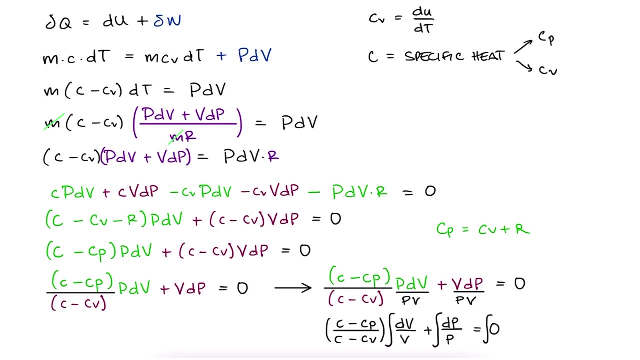 we can substitute these terms by a Cp. We can now divide by C minus Cv to have a coefficient next to Pdv and also divide all terms by Pv. Since the coefficient of Cs is constant, we can integrate with those terms outside the integral to get the parentheses. 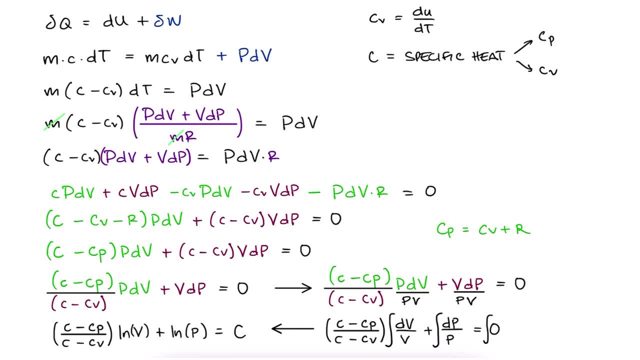 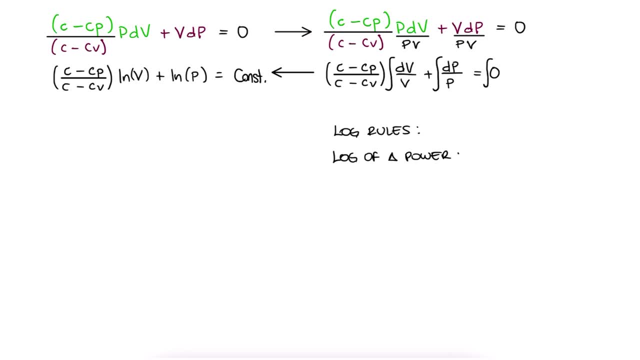 times natural log of V plus natural log of P, equal to a constant. If you remember basic exponentiation and log rules, you might remember the log of a power rule where Y- natural log of X- is the same as natural log of X to the Y. We can therefore write the first term as natural log of V. 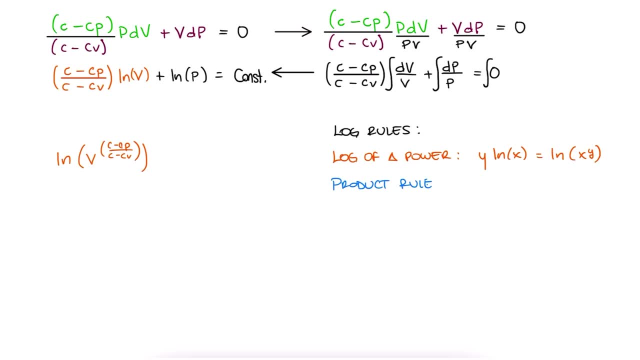 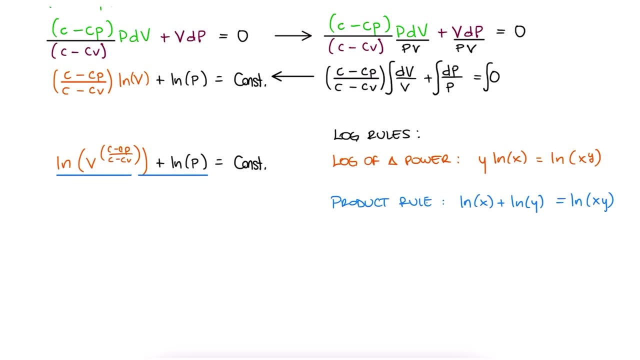 to the parentheses, And you might also recall the product rule where natural log of X plus the natural log of Y is equal to natural log of XY. This means that the left hand side is the natural log of Pv to the parentheses and therefore this is equal to a constant. The parentheses is what. 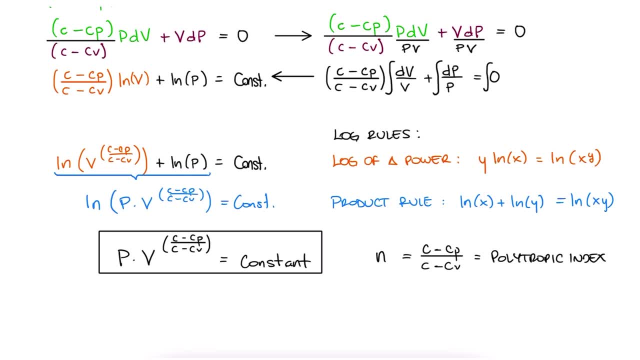 we call the constant N the polytropic index and therefore for a polytropic process of an ideal gas, Pv to the N is constant. This also means that P1, V1 to the N is equal to P2, V2 to the N, equal to P3. 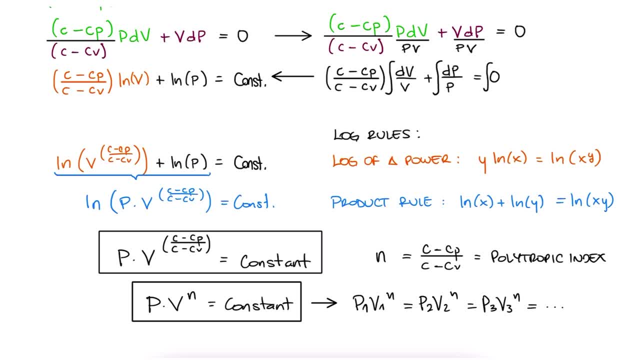 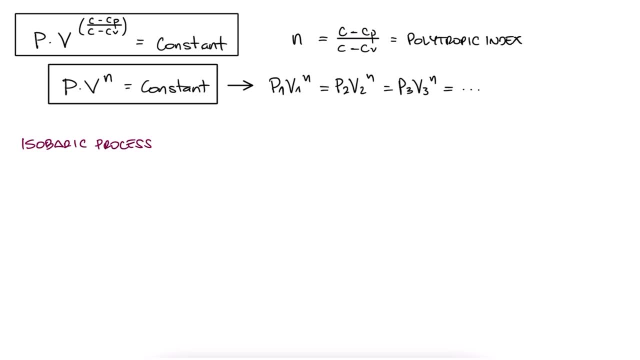 V3 to the N, etc. We'll take a look at other cases in just a second. but what happens if we try to apply this equation to an isobaric process? An isobaric process, or in other words, a process at constant. 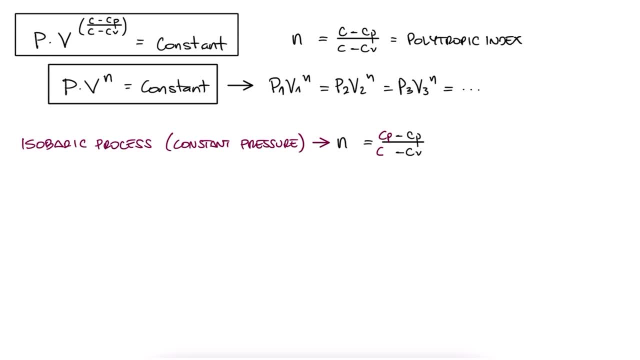 pressure means that our general specific heat C is Cp. This would mean that N is equal to zero. What about an adiabatic process, meaning that no heat comes in or out, In this case, since dq is zero and temperature changes can still occur? we would say that Cp is equal to zero. So what about an adiabatic process, meaning that no heat comes in or out? In this case, since dq is zero and temperature changes can still occur, we would say that Cp is equal to zero. 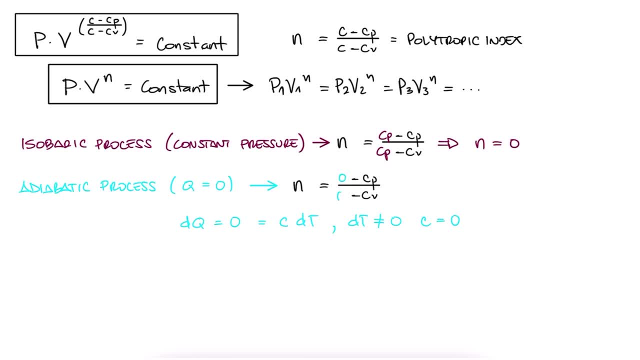 So what about an adiabatic process, meaning that no heat comes in or out? In this case, since dq is zero and temperature changes can still occur, we would say that Cp is equal to zero. Substituting this zero, we see that N becomes Cp over Cv or k, the specific heat ratio that 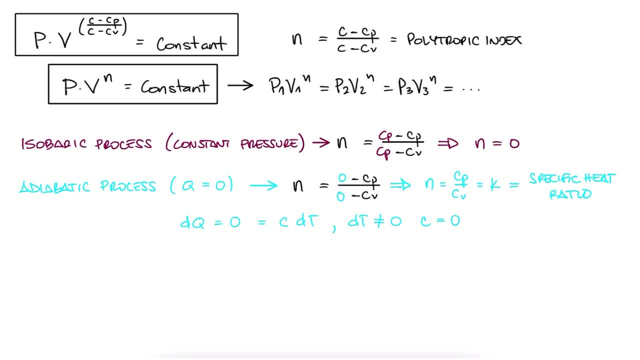 we established in the previous lecture. For adiabatic processes, this equation becomes Pv to the k equals constant. For an isochoric process, constant volume- we would have the general C be Cv, the specific heat at constant volume. In this case the denominator would approach zero and therefore N would approach infinity. 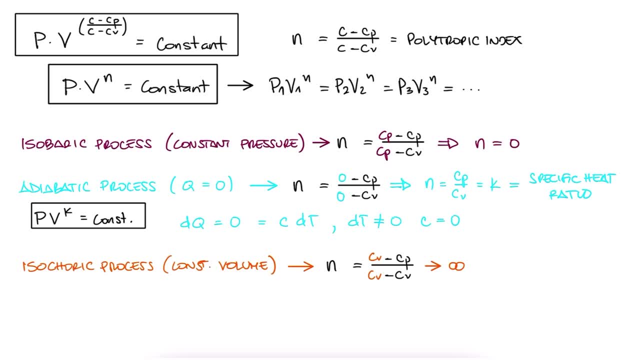 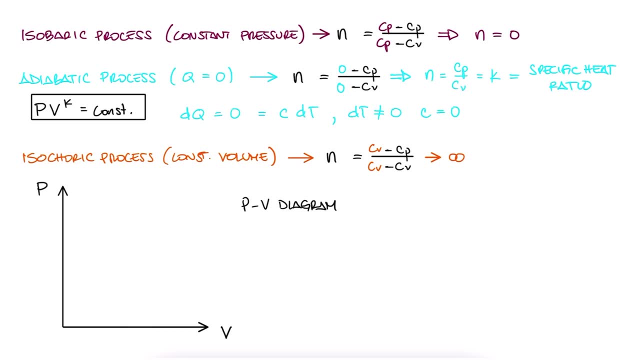 In this case, the denominator would approach zero and therefore N would approach infinity. This is not very useful in terms of solving for values, but it does allow us to plot these processes in a Pv diagram, where P is on the y-axis, v on the x-axis and for N equal to zero. 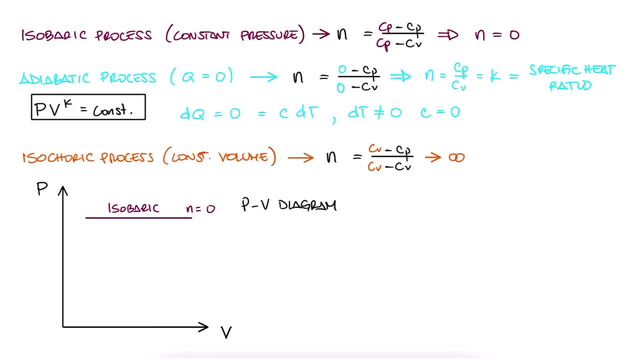 isobaric process. the slope is zero. N equals infinity, is an infinite slope or a vertical line, and an adiabatic process has a logarithmic slope equal to k. The first two make sense. N equal to zero is isobaric, meaning that the pressure never changes. 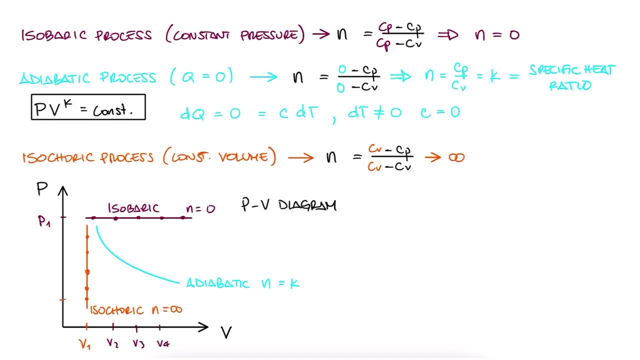 and N equals infinity is an infinite slope or a vertical line, and an adiabatic process has a logarithmic slope equal to k. N equal to infinity is isochoric, meaning that the volume is always the same. We'll look at an isothermal process in just a second. 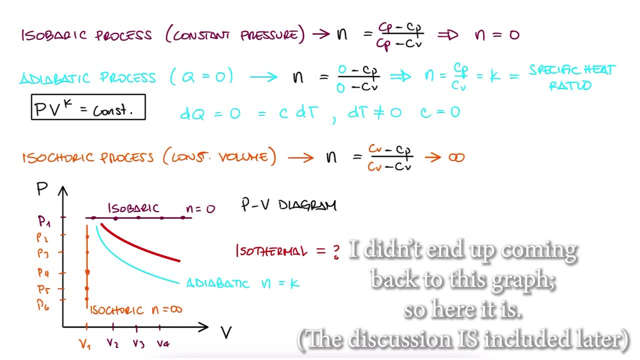 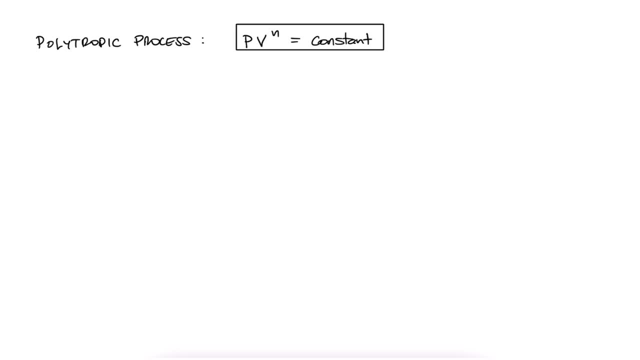 Just remember that, depending on the path from state 1 to state 2, the shape of this curve can be described by different values of N. The reason we use this relationship is because we need to know P in terms of v so that we can integrate Pdv and calculate work. 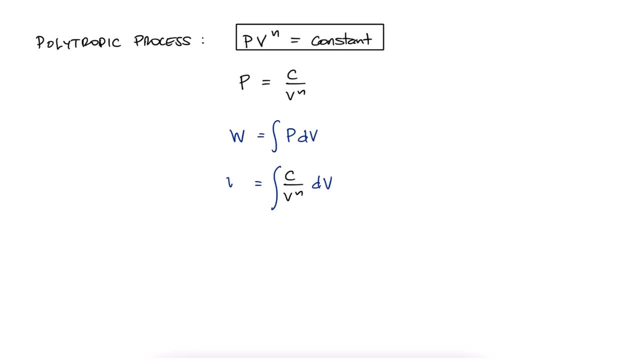 Substituting P in terms of v in the integral looks like this: or with the v in the numerator and the constant outside of the integral, we get v to the minus N. After integrating this expression, we find an equation for w in terms of the constant C. 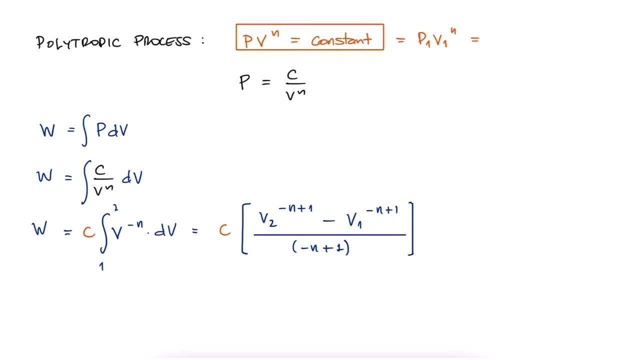 And since the constant is P1v1 to the N or P2v2 to the N, we can distribute it in our expression and substitute it for P2v2 to the N in the first term and P1v1 to the N in the second term and use the product exponentiation rule to find the expression. 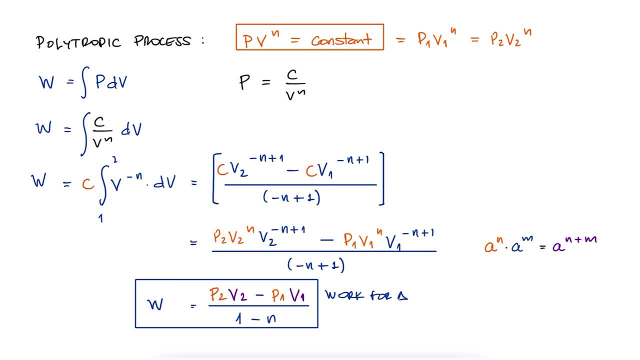 for work of a polytropic process in terms of P and v only. This expression is only true for N different than 1, and not because we would run into some mathematical issues dividing by zero, but because if N had been 1 from the beginning, 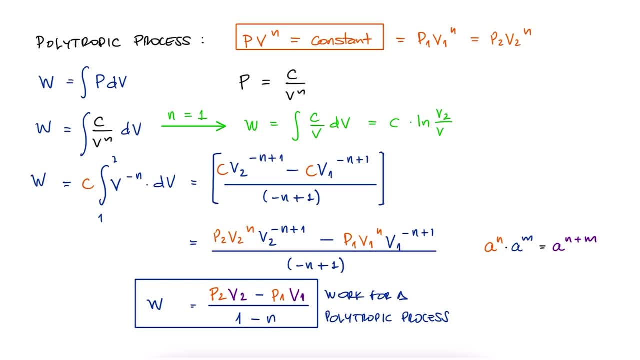 the integral would have been the natural log of V2 over V1 times C, in this case PV. This is the expression for work of a polytropic process when N is equal to 1.. And notice that P and v can be that for any state. 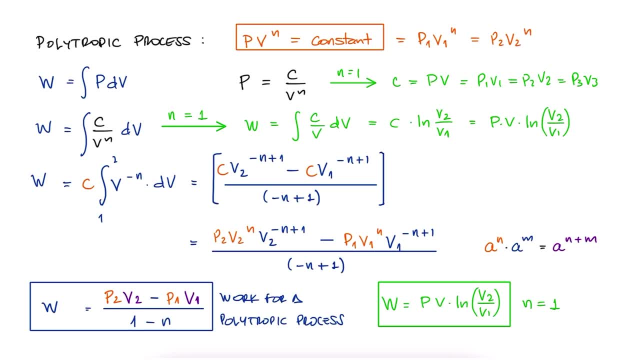 P1v1, P2v2, P3v3,, since the constant is the same for any state. And what does it mean that N is equal to 1?? Well, if P1v1 is equal to P2v2, from our ideal gas equation, this is only true if the right hand side 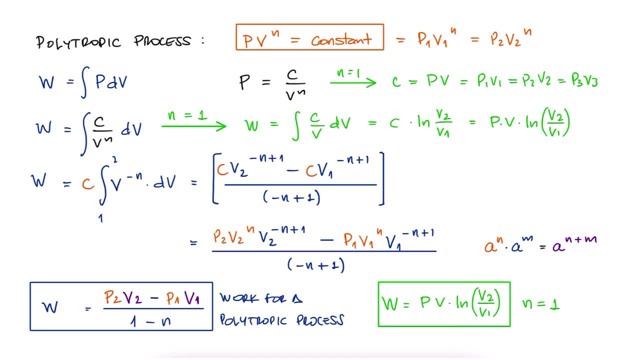 of the P times V equation is constant. The right hand side is R bar T1 for the first one and R bar T2 for the second one. If these two are equal, it means that T1 and T2 are the same. Therefore, the big conclusion here is that when an isotropic index N is equal to 1,. 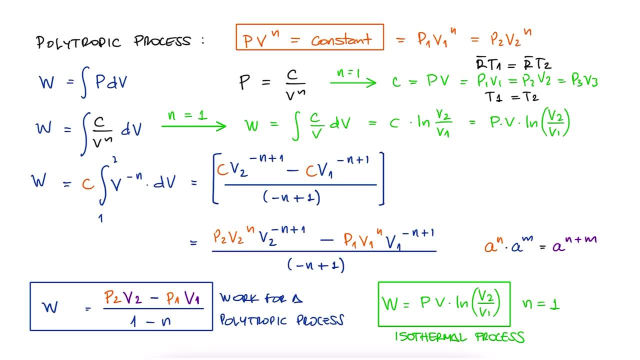 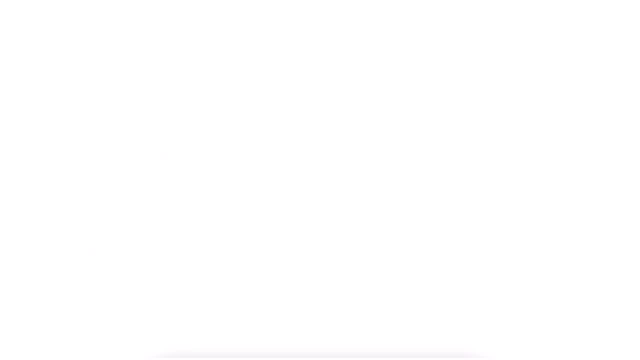 the process is an isothermal process or a process where the temperature is kept constant. Let's make use of these expressions with a simple example, and if you want to see more complex examples, make sure to check out the videos for this topic in the description below. 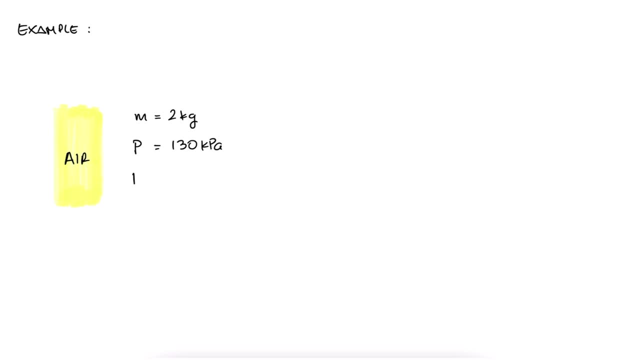 2 kilograms of air at 130 kilopascals and 22 degrees Celsius is contained within a piston cylinder Press to a final pressure of 550 kilopascals. During compression, heat is transferred from the air and the temperature remains constant. Determine the work input required using a 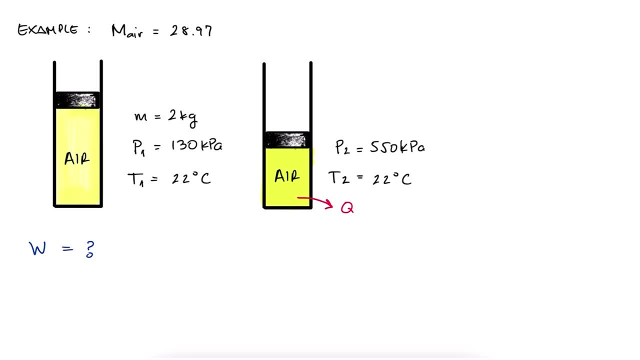 molecular mass for air of 28.97 kilograms per kilomole. As always, pause here and try to solve this problem before watching the solution up next To solve for the work we know we have two options we derived today. One for when the polytropic index is not 1,. 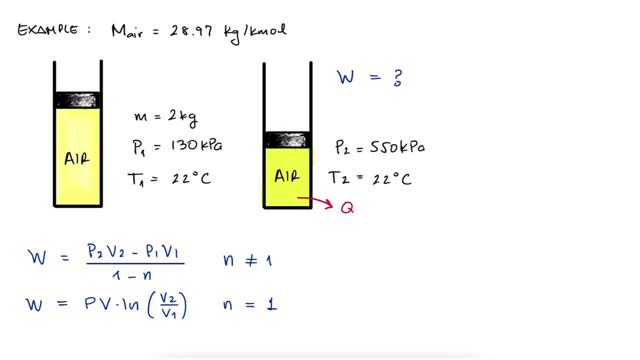 and one for when the index is in fact 1.. And since we're being told that the temperature remains constant, meaning an isothermal process, we know N is equal to 1.. We have P1,, P2, and T1, and again we are trying to find the work. 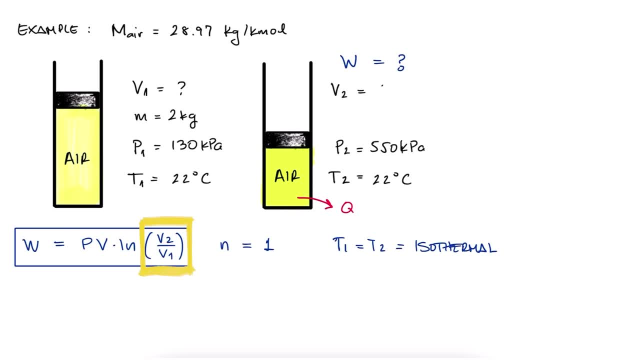 which from these equations we see that we first need V1 and V2.. To find V1 first we can multiply the specific volume V1 times the given mass, and to find V1, we use the ideal gas equation. Remember to use the ideal gas equation. 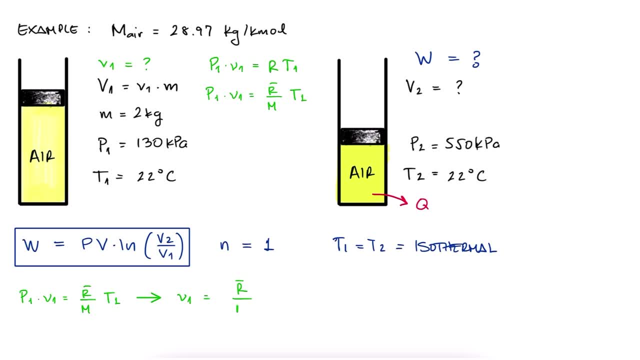 Remembering that R is R bar over M, with M for air, and that temperature has to be input in Kelvin, not Celsius, we substitute the pressure to find the specific volume of state 1 in cubic meters per kilogram And, like I said, since we're given the mass, we find V1. 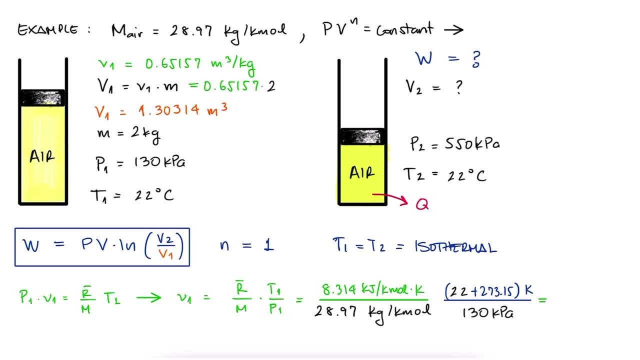 Now, since we do know that N equals to 1,, then P1V1 is equal to P2V2, and therefore V2 is equal to P1V1 over P2.. With this we can find the volume at state 2.. 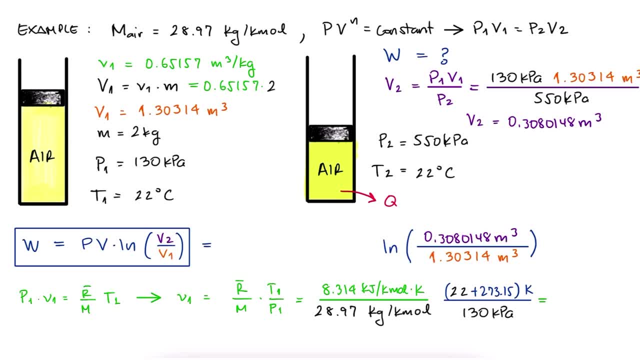 And finally, we use the expression for work that we derived today, and it doesn't matter if we use P1V1 or P2V2 here, Since N is equal to 1, they are both the same. This negative value we get for work is consistent with what we know about heat and work. 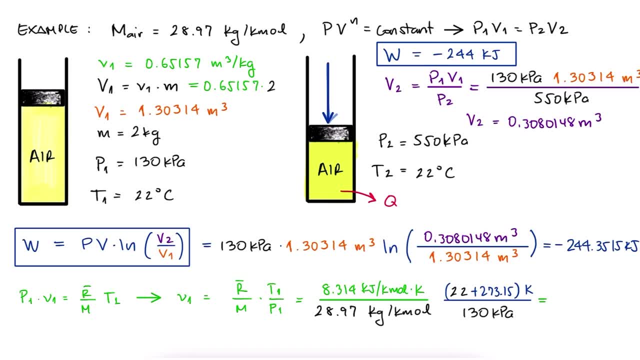 Since this is a compression process, we need to put work into the system to compress it, and our convention was that work in must be negative. If you want to check out other examples on this topic where we use the other expression we derived here today, or the other lectures of the thermodynamics course and lectures, 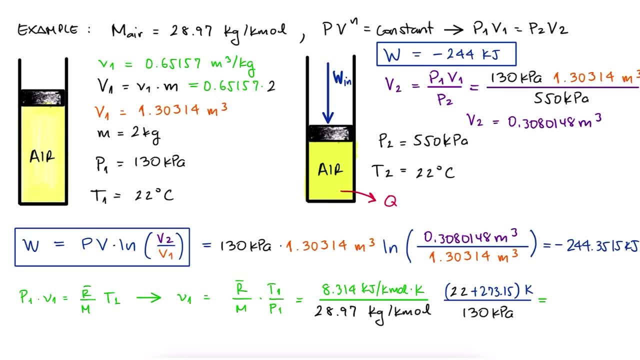 of other engineering courses. make sure to check out the links in the description below. Thanks for watching.